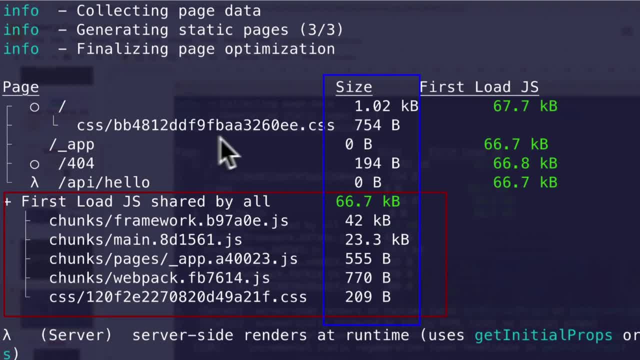 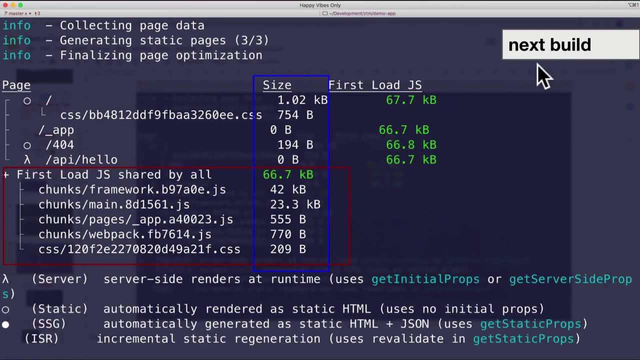 to do Now? on the left-hand side, it essentially lists all the pages that we are basically using. At the bottom, it has divided all those different pages into different chunks. Then we have the size column and the first loadjs. Now next build creates an optimized production build of your application. 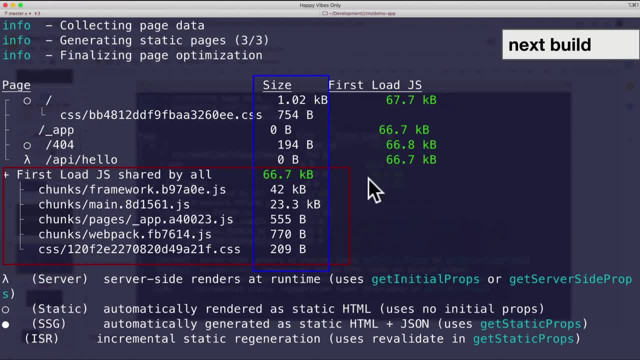 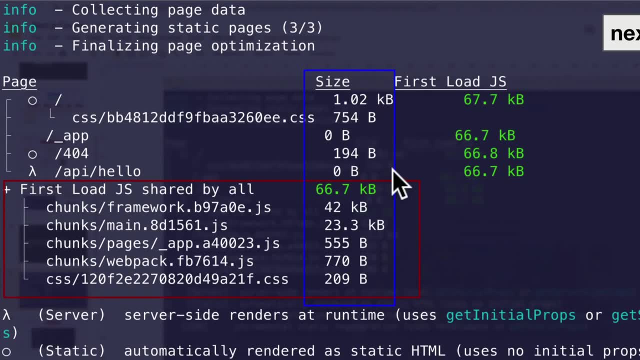 The output of this is something you would upload on your server and deploy it to your domain. Now, the size column indicates the number of assets downloaded when navigating to the page on the browser, And this is essentially the size of every route, including the dependencies that. 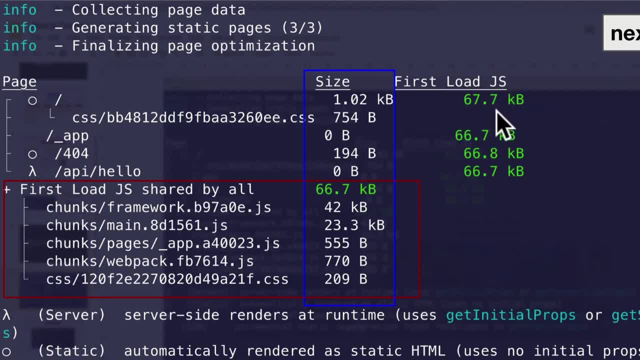 every route uses, And the first loadjs is the number of assets that we are going to use, number of assets we download when visiting the page from the server as well. Now this specific red box indicates how Nextjs has performed code splitting. These are different chunks that we were just talking about. 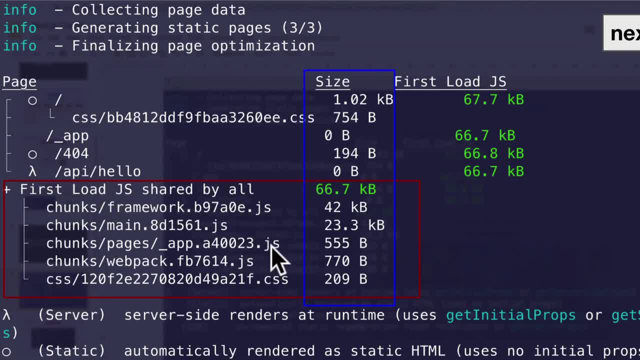 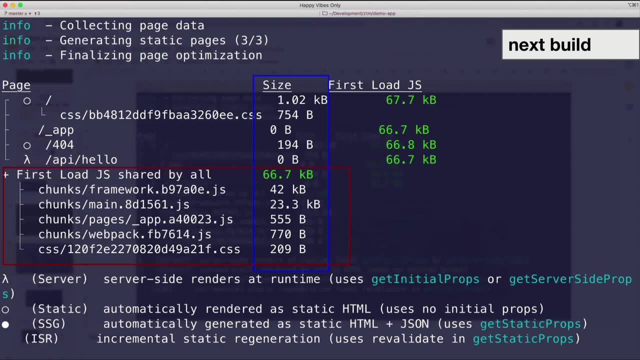 It is basically the first load JS that is shared by all. The Nextjs is only going to download that specific bundle or chunk that is used by that specific page. It is not going to download content for the entire website. if you are never going to visit, 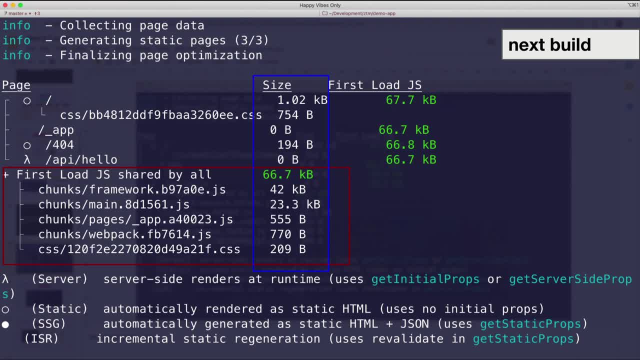 it. Next thing that Nextjs also does is code minification, And minifying code essentially means that Nextjs is going to get rid of all the special characters, white space and so on, to make the file size really tiny. This is one of the techniques that it uses to shrink the file size. 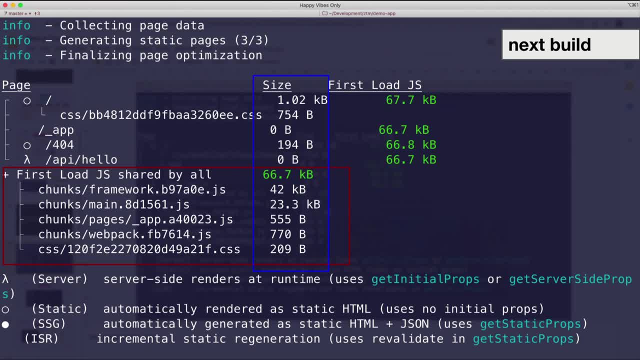 Now Nextjs minifies the code for you, So you don't need to do that yourself And your files that get packaged to the browser are really small and therefore you get a huge performance boost because of that as well. Now, if you do remember, in create react app we had to do code minification using webpack. 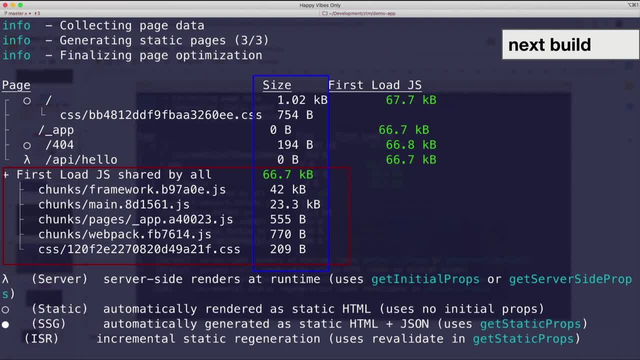 separately And we had to learn all of that. Learning webpack and mastering webpack is not easy and that is definitely a skill that we need to master when we are using Nextjs. But this does not mean that we should not care about how webpack works and some of the 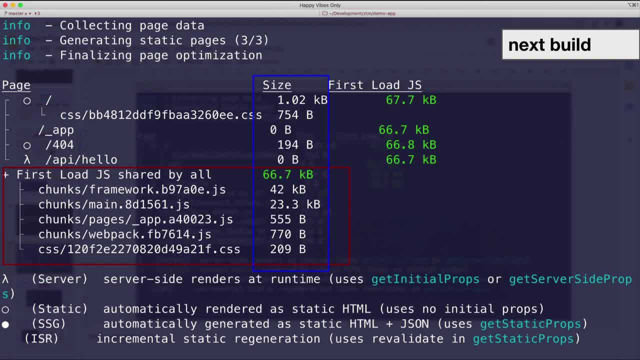 domain knowledge related to performance. These are important concepts that you need to learn. as a developer, You definitely need to know what they are and how they work, But in my opinion, a lot of fatigue while building react application comes from having a lot of choices. 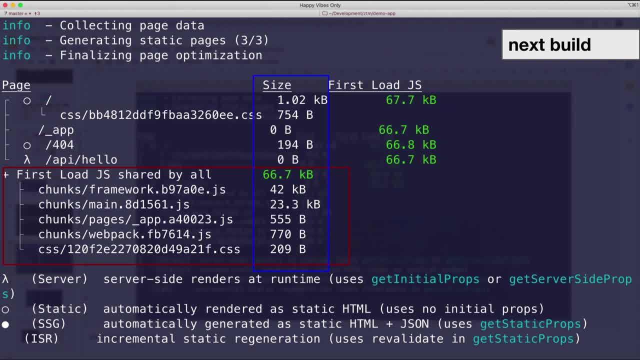 And in Nextjs It is taken care of a lot for you. So you need to know what the concepts are and how they work, But Nextjs takes care of it for you. So you are offloading the burden to a framework, a popular framework that has a really good 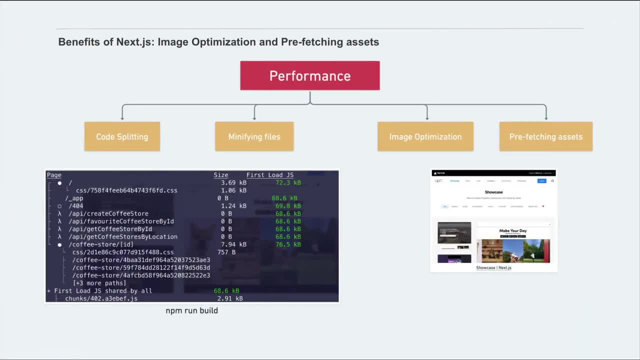 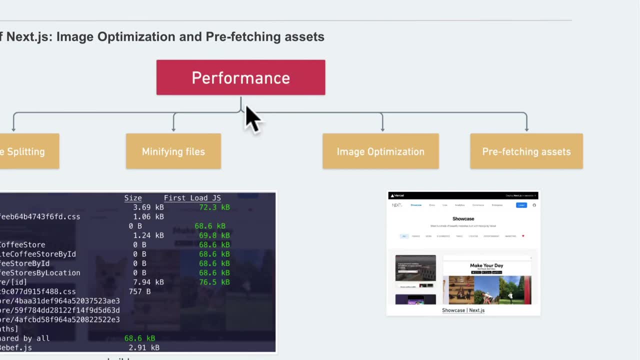 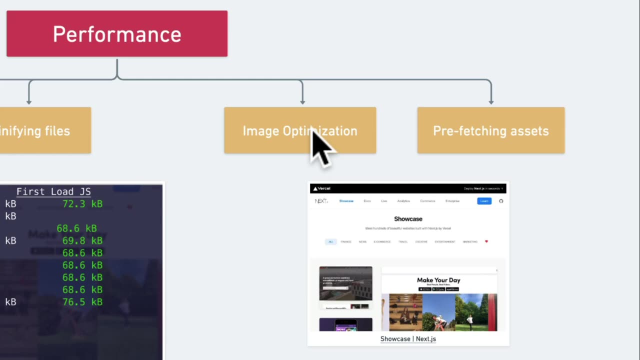 developer community. Now, next, let's take a look at image optimization and prefetching assets, which is another thing that helps with performance with Nextjs. Now, Nextjs Starts us with a few components out of the box. One of them is a next image component. 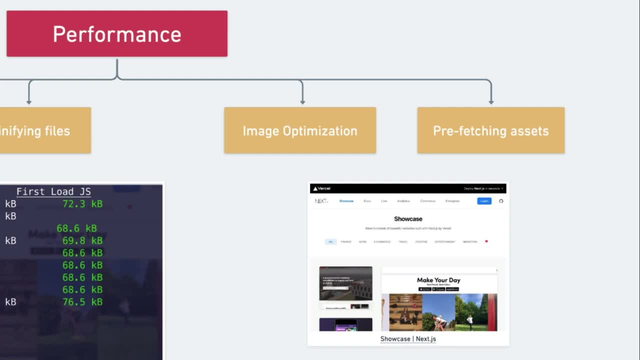 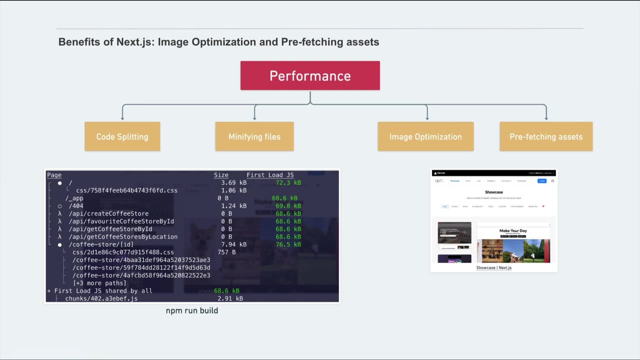 Now, images are going to be automatically optimized for you with this specific component. Now, if you imagine, our web has a lot of images. Our sites have a lot of images on them and they make up for a lot of the performance as well, So it's extremely important that these images are performant. 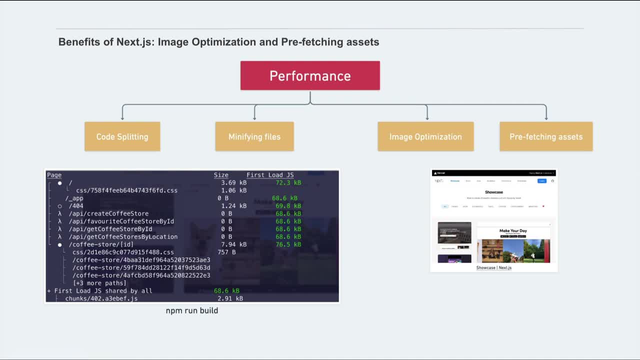 So our site can load faster. Now in Nextjs, instead of using the image tag from the browser, we will essentially be using the image component from Nextjs, And Nextjs will serve an image based on the browser size, So if you're on a mobile device, you will see a smaller image. 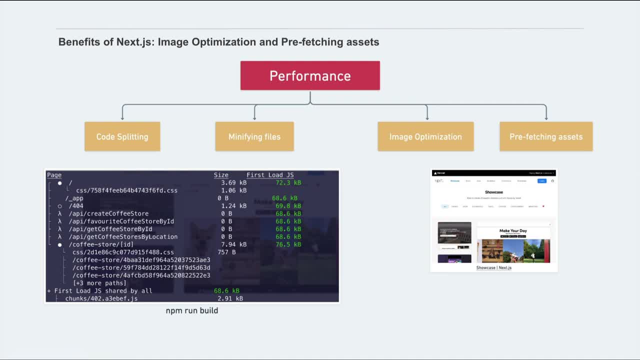 Instead, if you are on a desktop, then you essentially see a much larger image. So, based on your browser, Your browser window size or based on your device type, it is automatically going to serve that image for you, And all we need to do is use the next image component. 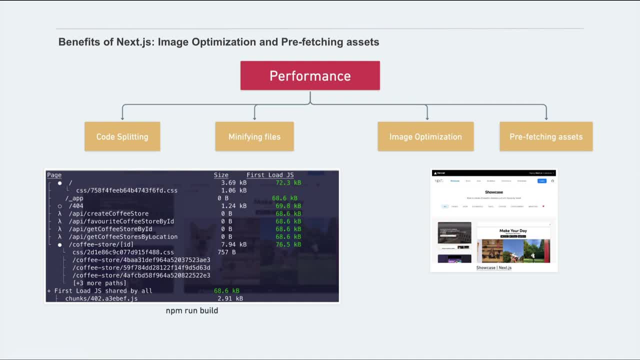 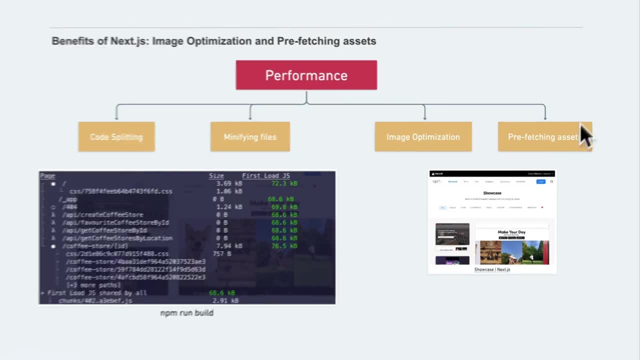 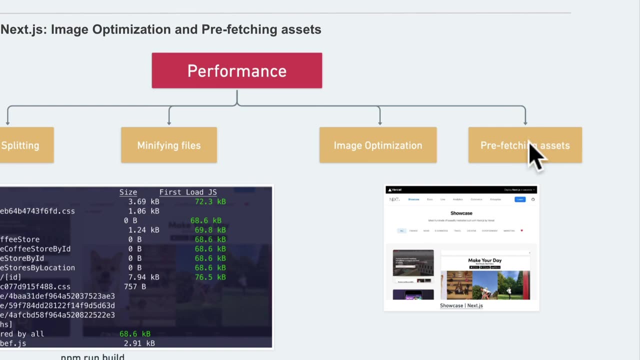 Now, isn't that amazing. Next image component provides us with a lot of cool features as well that we will take a look at later in the course, Such as prefetching assets. Nextjs only will go ahead and prefetch specific assets as you scroll down the page. 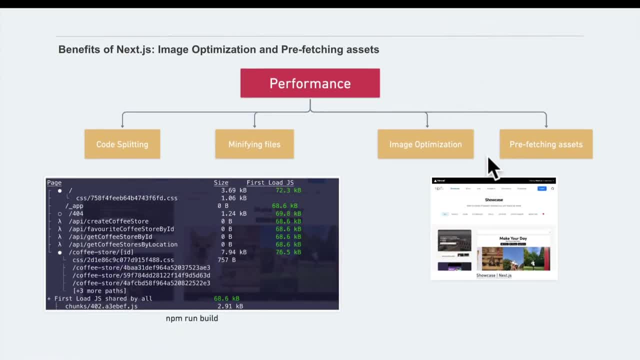 So Let's take a look at how images work in a demo with images next. I'll see you in the next one.